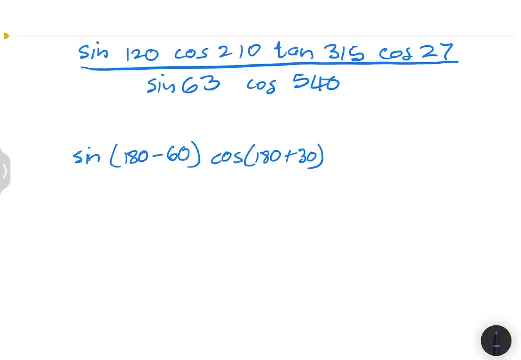 so, as much as it's possible, I'm going to try and use 180 and 360.. OK, Remember that once you change to 90 and 270, we change to code ratios Right, So now we've got 10 of 315.. That would be. 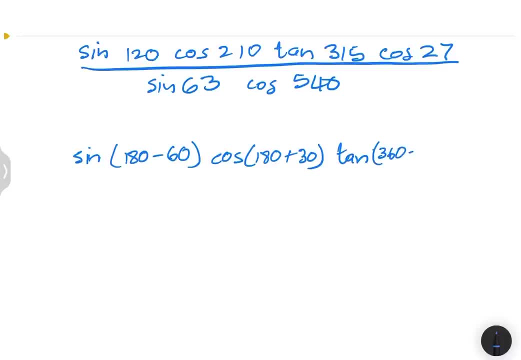 the same as 360 minus 45.. OK, And of course now, if you look at this cos of 27, you always need to look at the smallest angle that you have, So in this case, I'm going to leave this exactly as it. 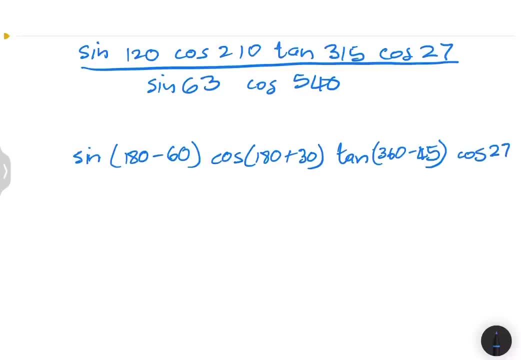 is because it's not part of our spectrum. So I'm going to leave this exactly as it is, because it's a special angle Right, And in this case now I see we've got sine of 63. So it's not a special. 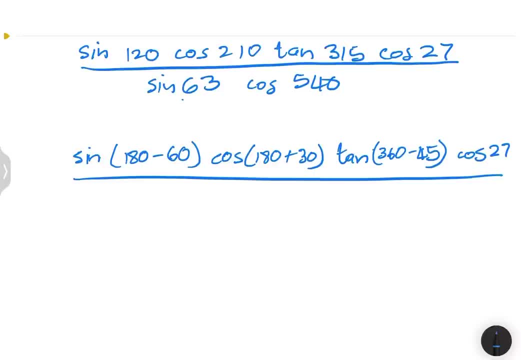 angle as well. So what I'm going to do is I'm going to leave it. In fact, I'm going to try and write it in the form of that small angle that we have there. OK, so when I look at sine of 63,, 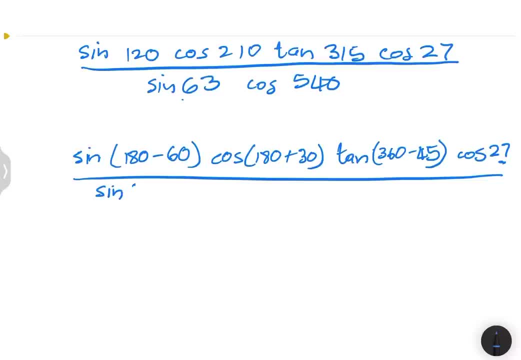 you'd agree with me that this would be the same as sine of 90 minus 27.. Right, 90 minus 27 does give me 63. And the reason I'm changing it is so that it can look like that other angle there, Right? So remember, you take the cube from the smallest angle that you. 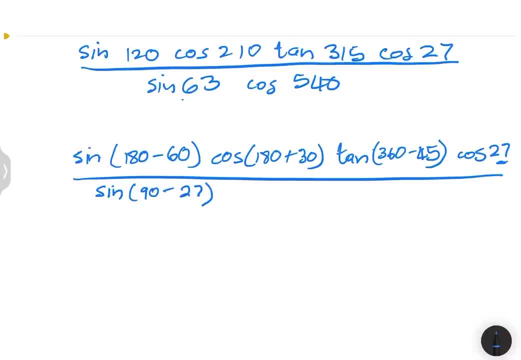 have. That is not part of your special angles, Right? So in this case I'm going to have cos of 540.. If you want to cos of 540, that's quite big Right. So in this case you could have. 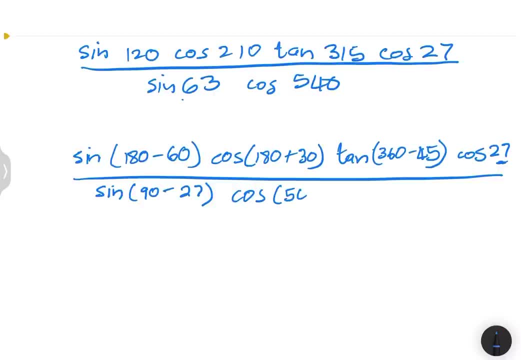 cos of 540 minus 360.. Now, remember, 360 is the repetition in this case, That's the. you know the interval in which any repetition takes place. So, as a result, you can either add 360 or subtract 360.. You know, your angle still remains the same. All right, Now let's, let's try and use reduction. 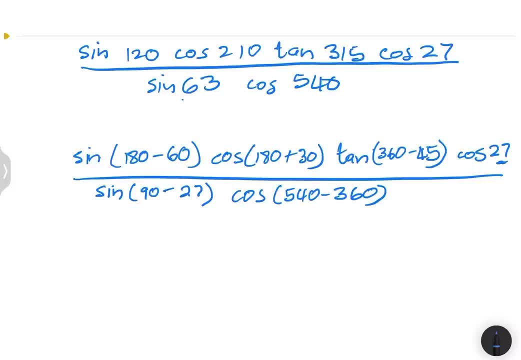 formulae here. So we're going to say sine of 60 minus 360.. So we're going to say sine of 60 minus 180 minus 60. Remember how is sine? So we use a cast diagram. Okay, So 180 minus 60. Remember. 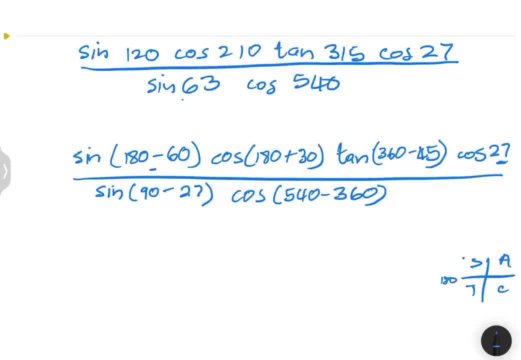 180 is over here minus 60. So that would be in the second quadrant Right. How is sine? in the second quadrant? Sine would be positive, So this would be sine of 60.. Okay, And we've got cos of. 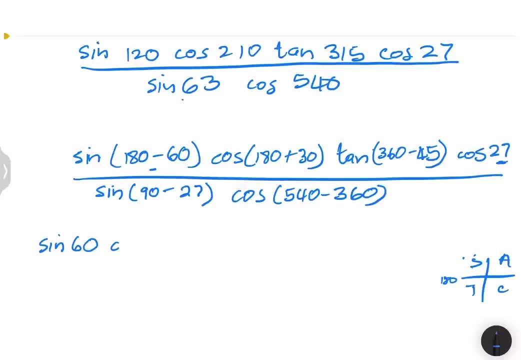 180 plus 30. Now, cos of 180 plus? that's 180 minus 60. So we're going to say sine of 60 minus in the third quadrant, Right? So how is cos in the third quadrant? That would be negative, So this: 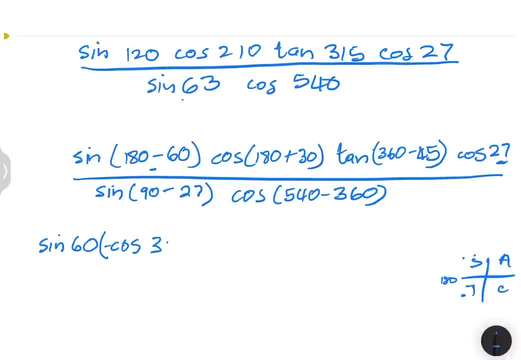 would be negative. cos of 30 degrees, Okay, And we've got 10 of 360 minus 45.. Okay, We'll look at that. It's in the fourth quadrant. How is 10 in the fourth quadrant? It's also negative. So 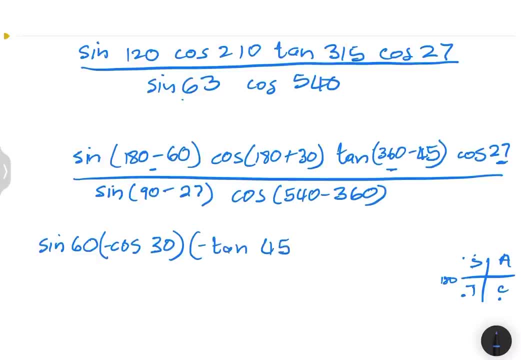 that would be a negative 10 of 45. And we've got cos of 27.. As I did say, I'm going to leave it in that format. All right, All of that over Now. in this case, we've got sine of 90 minus 27.. Now, remember 90 minus. So that would be in the first. 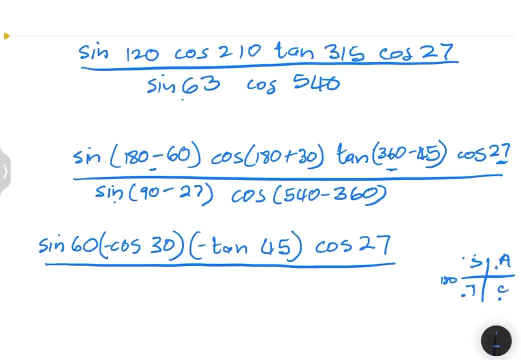 quadrant. All of them are positive. All of my ratios are positive there. So in this case I'm going to say, well, sine of 90. So that's going to be positive, But remember, when we use 90,. 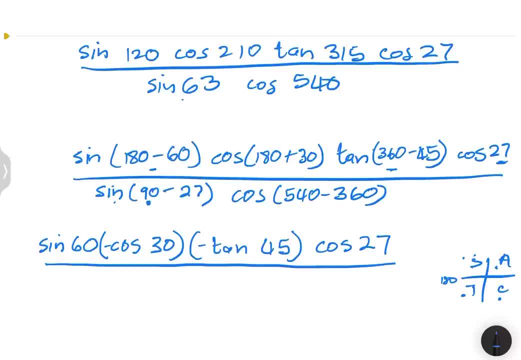 we are going to change to our co-ratios, Right? So in this case that's going to be the cos. Remember, the co-ratio of sine is cos, Okay. Or the co-function, in this case, of sine, is cos, So that's cos of 27.. Okay, And that would be cos of. now, if we take 540 minus 360, in this, 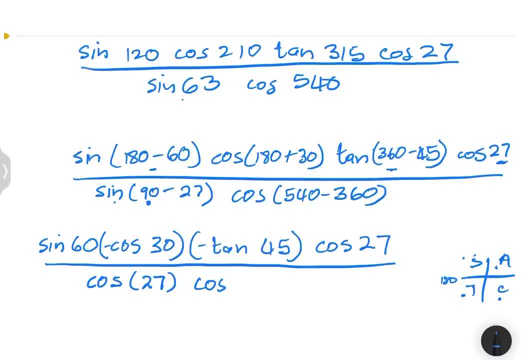 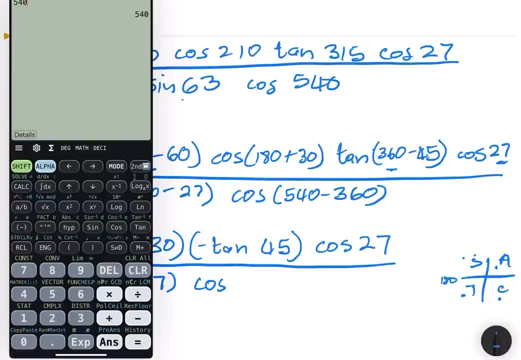 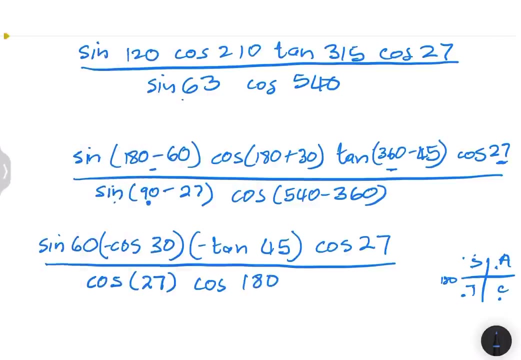 case, that would give us 180.. Right, So, okay, let's verify that so that we make sure. So that's 540 minus 360.. Okay, Yes, definitely it is 180.. So that's cos of 180. Okay, Right Now, let's use our special angles in this. 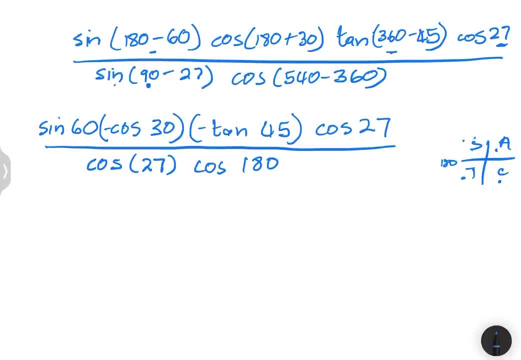 case. So we've got sine of 60. And remember, when we use special angles, in this case, we always need to be mindful What are special angles. We always need to be mindful of what are special angles look like. Okay, If you haven't watched my longer video on this section, please have a look at it. So 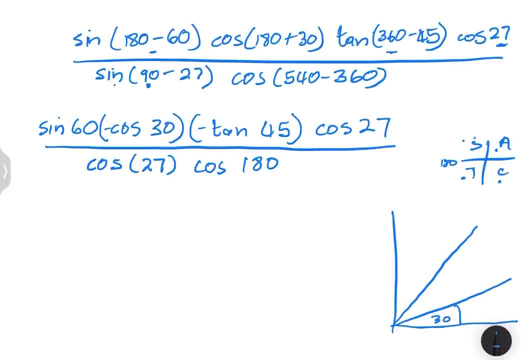 we've got 30.. We've got 45.. Okay, so, let me just remove this one. Okay, So we've got 30.. We've got 45.. All right, we've got 60. And we've got 90.. Okay, which is that one over there? All right, And 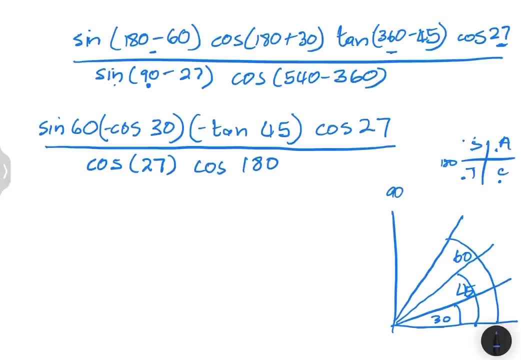 in line with row. Now those effects times are 30 times what we've set the interval for today. The way that we look at this is we're gonna look at all the various events Now. the number of the events are the number of times, and so this is the number of times: 1,, 2,, 3 times, 1 times 3 times. 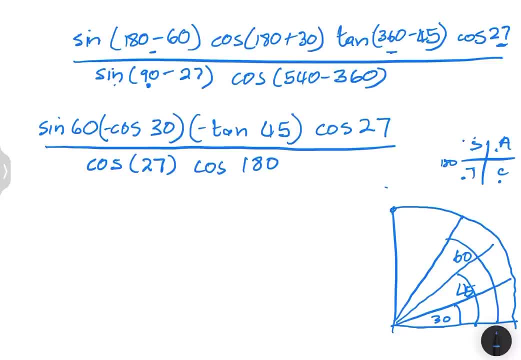 3 times is the number of times the event takes place. So w and 1 equals y. So you'd be aware that this is not a straight line. So we have a 1999, see, we have aematide and a 20 Ji, Anything else. 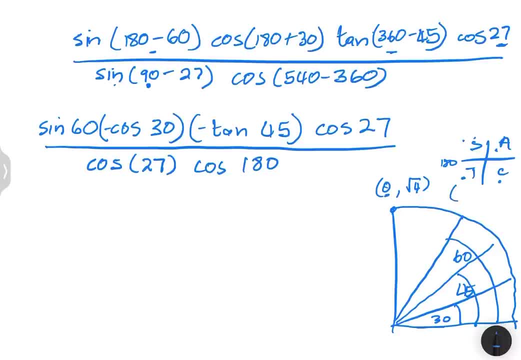 き. Now let's start with the X. It's going to be 0, that's square root of 1, square root of 2, square root of 3.. As I said, yeah, maybe let me just try and move it away from the corner here. 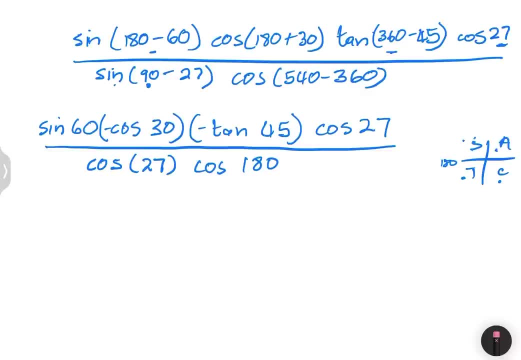 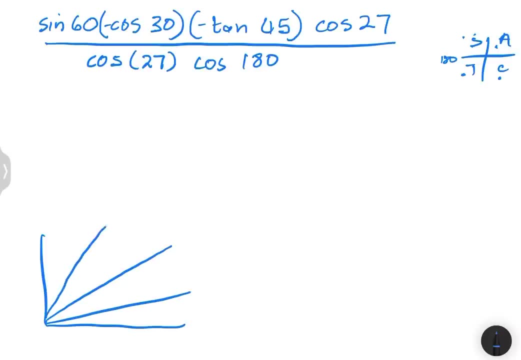 OK, I was trying to get it as far away from the main thing that I'm doing. OK, so in this case, as I said, OK, so there you are. You've got a circle that has a radius of 2.. 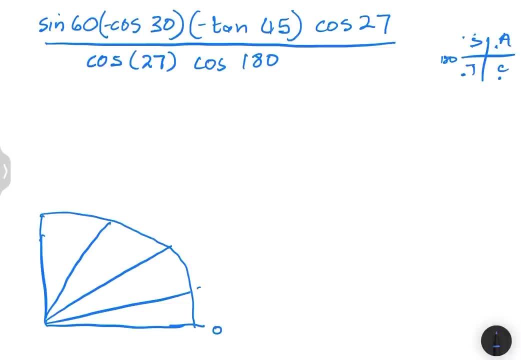 We have 0 degrees there, We've got 30 degrees there, We've got 45 and we've got 60 degrees and 90 degrees. Right Now the easiest thing to get the coordinates there Right I start. I know that my X here is maximum. 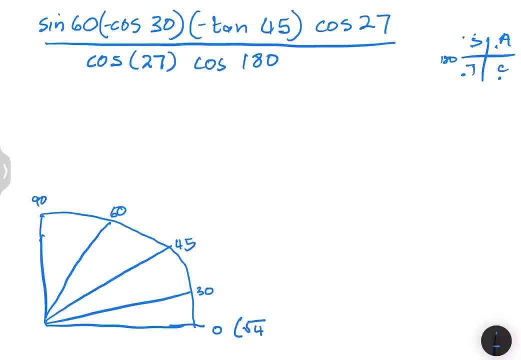 So that's 2.. So that will be root 4.. You say root 3,, root 2,, root 1.. And of course, root 0, which is 0. Right, And in this case I'm going to do the same for my Y. 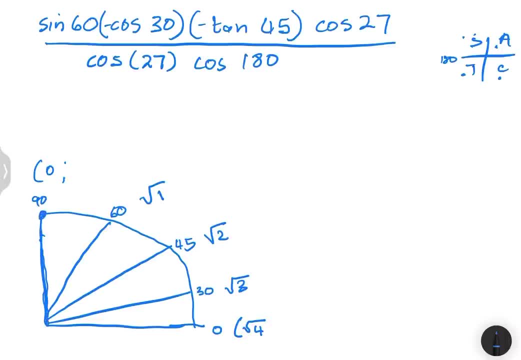 Remember that my the radius of my circle is 2.. So it means my Y value would be 2 there. So that would be root 4.. That's root 3.. That's root 2.. That's root 1.. And of course that would be 0.. 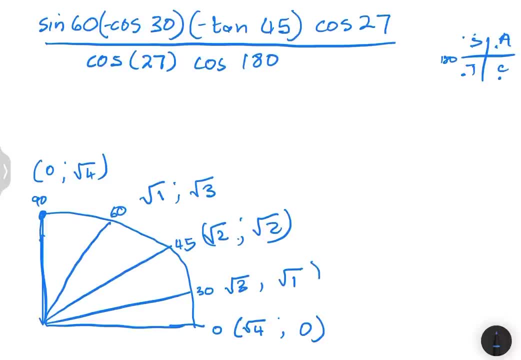 So that's how you remember your special angles. Now remember: the R value is always 2.. Right, So your R value is always 2.. The distance from the center there to the circumference, the radius Right Would be 2.. So it doesn't matter where you are, Your radius still remains 2.. 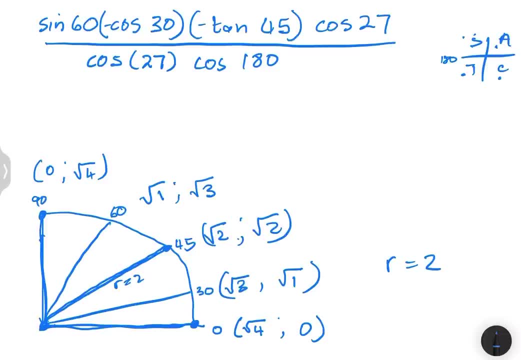 OK, Right, So let's apply our special angles in this case, Right? So I've got a sine of 60.. So, if I go to my special angles, the sine of 60 in this case. And of course, you guys, I know that you can cheat this by looking at your calculator- 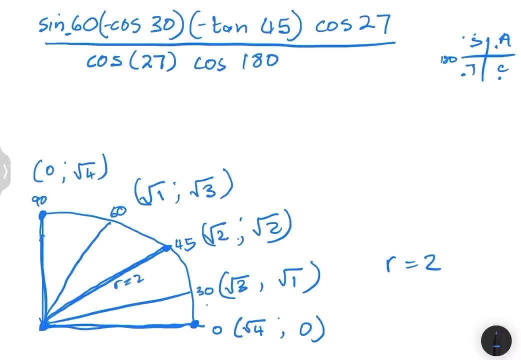 But I just wanted to show you how to apply it without using a calculator. Right, So, sine of 60. So remember that sine is Y over R, OK, Or you can say opposite over. So in this case that's Y, which is root 3, divided by R, which is 2.. 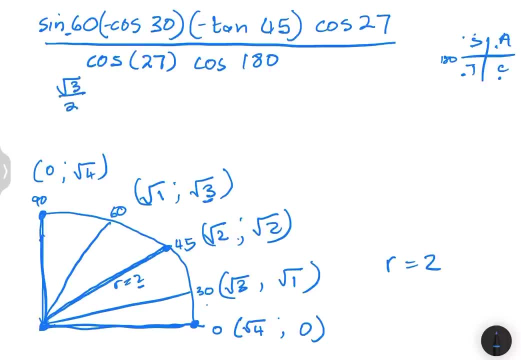 So sine of 60 is root 3 over 2, multiplied by negative cos of 30. So when I say cos of 30, remember that's X over R or adjacent over hypotenuse. So it's going to be X root 3 over 2 again. 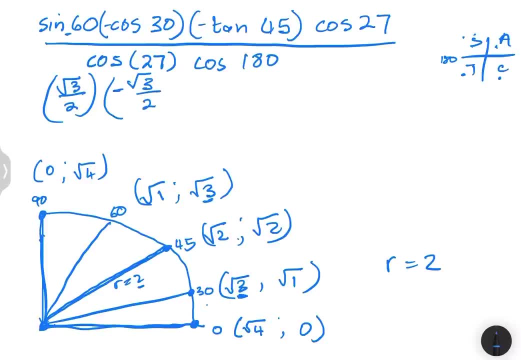 But remember it's. It's negative. So negative root: 3 over 2.. OK, Multiplied by negative, 10 of 45.. So 10 of 45.. I'm sure you guys would know that 10 of 45 is 1.. 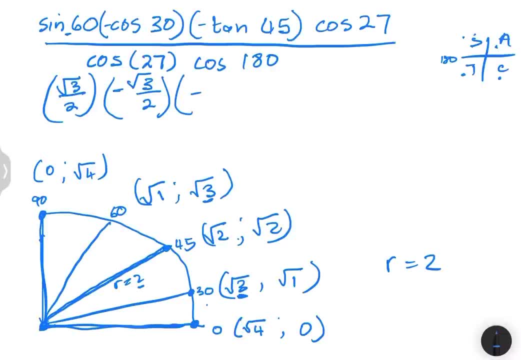 OK, But remember, it's Y over X. Why is it 1? Because my Y is root 2 and my X is root 2.. So that would be minus root 2 over root 2.. OK, And so, which gives us 1.. 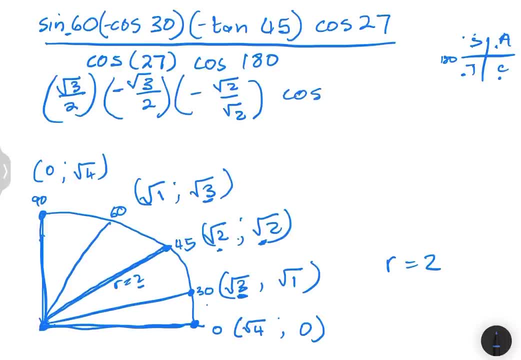 OK, Multiplied by the cos of 27.. OK, Right, So this is all divided by OK. Sorry that it looks a bit of a mess there. OK, So that's root 2 over root 2.. So this is all divided by the cos of 27..